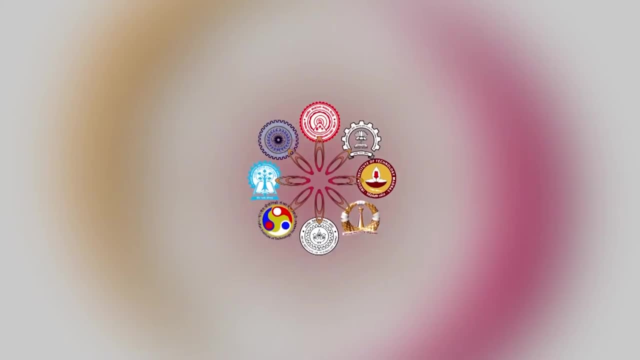 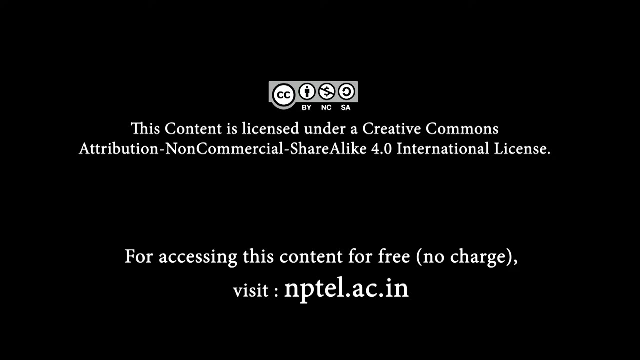 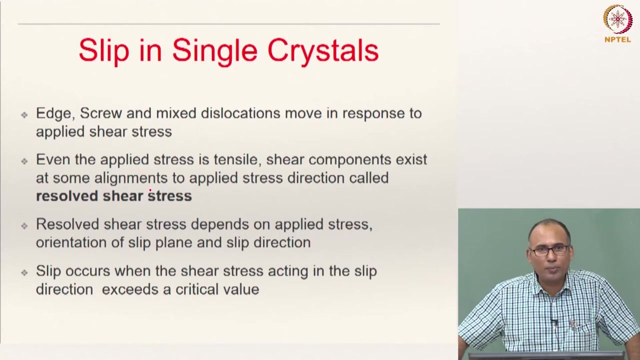 Now let us try to understand little bit more about slip in single crystals. So all that until now. what we have tried to understand is that materials will have line defects called dislocations, And the motion of these dislocations is what we call plastic deformation in crystalline. 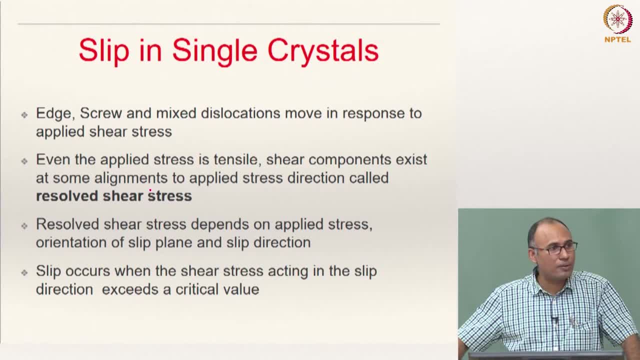 materials And these dislocations. whenever they move in a lattice- crystalline lattice- they prefer certain planes in which they want to move and then in those planes in certain directions in which along which they want to move. That means there are some preferred planes and preferred directions. In other words, they are also called slip planes and 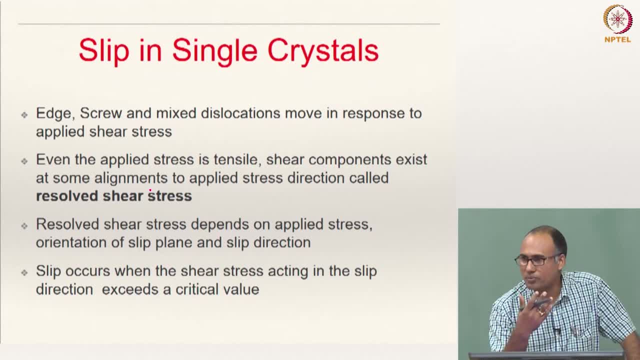 slip directions And together they are called slip system, right, So dislocations move in some preferential slip along preferential slip systems And the slip systems are different for different crystal structures And we have seen that FCC has 12 slip systems. BCC in total has 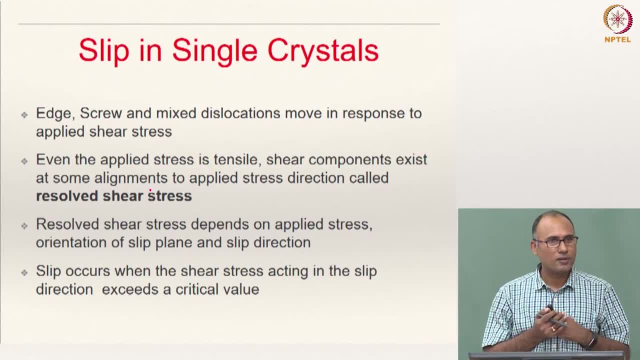 48, HCP also in total has 12 slip systems, And we have also argued that FCC materials are known to be more ductile compared to BCC and HCP. However, we did not answer the question why BCC, in spite of having larger number of slip. 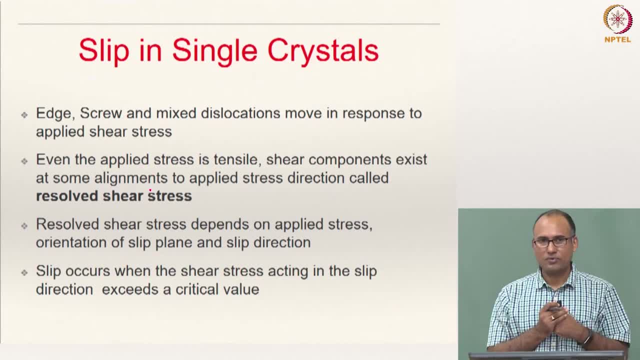 systems is less ductile compared to FCC right That we have not answered. That is something for you to think about. All right, Now we will move forward and try to understand a little bit more about slip in the single crystal materials. As we have discussed, we have three. 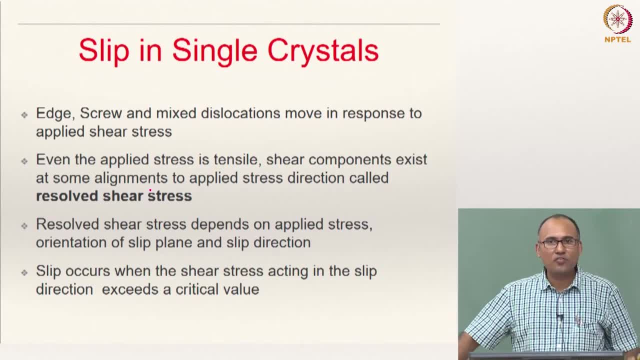 different crystal materials. We have three different kinds of dislocations: Edge dislocations, screw dislocation and mixed dislocations. When you subject this crystal lattice to external shear stress, then you apply shear stress on this lattice. then these dislocations tend to move within the crystal. 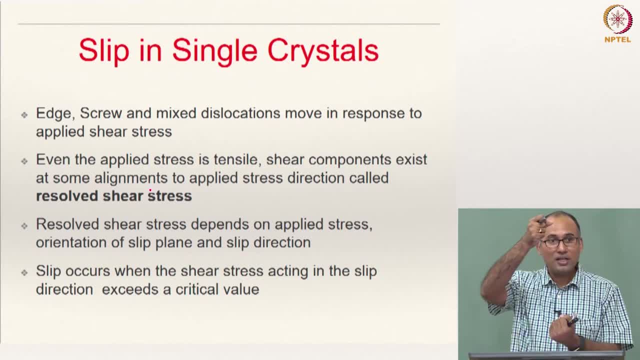 lattice, Even if the applied stress is tensile in nature, there are orientations along which you will have spring over the lattice. So this is that, So you have a performance, So you are also applying stress, So you require more stress, so you are able to shift é. 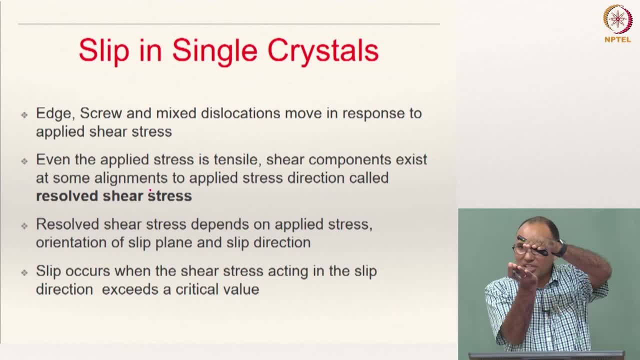 some shear, Because the plastic deformation is nothing but slip. that means shearing of one plate of atoms with respect to other plane of atoms. So if you are applying load like that, they are not going to slip. But these planes may not slip, this load might eventually. 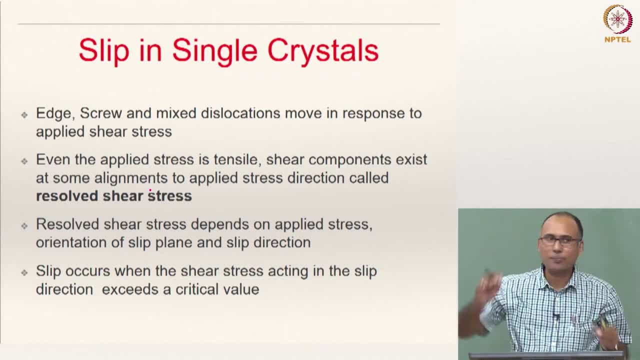 become effectively a shear stress on some other plane. that is what you have learnt through your Mohr's circle. If you know your shear stress, the loading applied in a particular direction, and then you can draw Mohr's circle and then identify in other planes how the 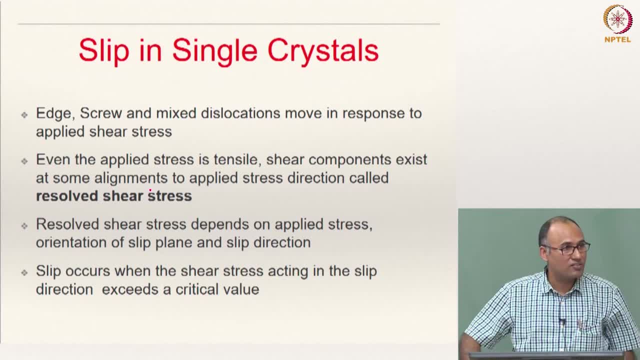 stress state is, And you can actually identify planes along which it is pure shear. only shear stresses remain. there are no tensile stresses. That is what you have learnt in your strength of materials class. the same applies here too. So even when the applied stress is tensile, shear components exist At some point in the 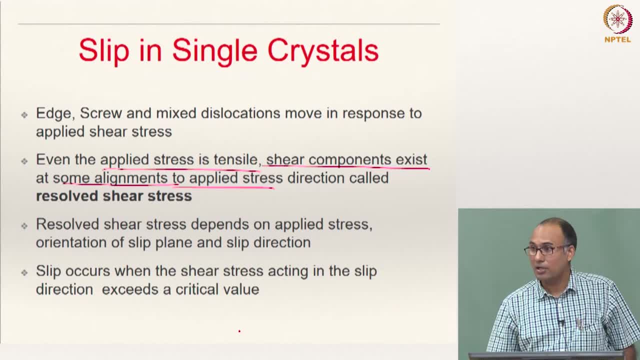 system, shear components are kept in a particular direction and then the shear stress is drawn in a particular direction. So you can see that there are some orientations or alignments to the applied stress direction and that shear stress is called resolved shear stress And the slip happens due to that resolved shear stress. So the real resolved shear stress. 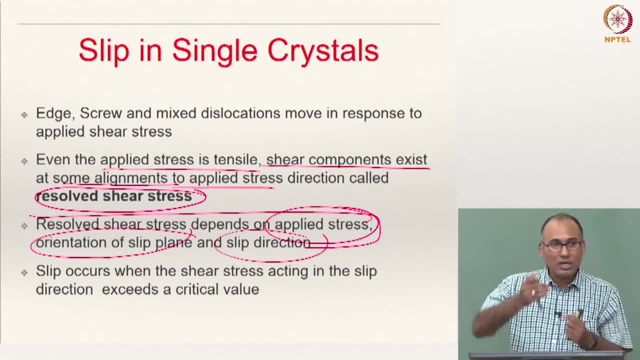 depends on what Applied shear stress and the orientation of this slip plane and the slip direction to the applied loading. if you want to calculate what is the resolved shear stress, it should depend on the magnitude of the load that you are applying and orientation of this load with respect to the slip plane. 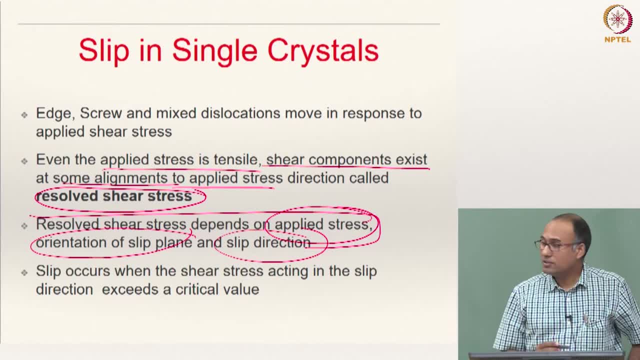 and the slip direction. So then slip occurs when the resolved shear stress acting on the slip direction, acting in the slip direction, exceeds a critical value. That means it should be able to break the bond. So that means the material will have some resistance, some 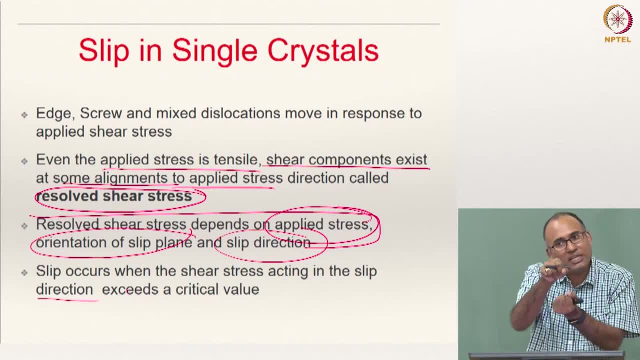 strength. The resolved shear stress should be able to overcome that strength. only then the slip will occur. Otherwise the slip will not occur. Otherwise you will only be causing elastic deformation. If you want to break the bond, you need to apply sufficiently large. 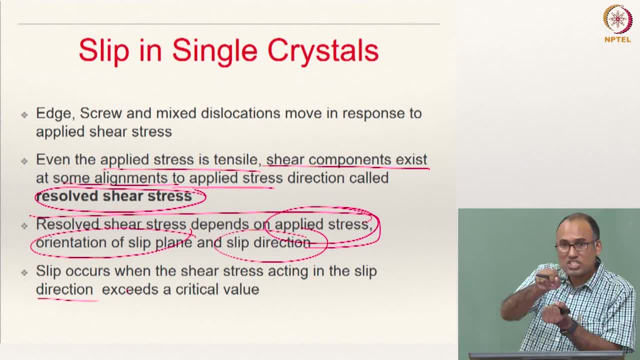 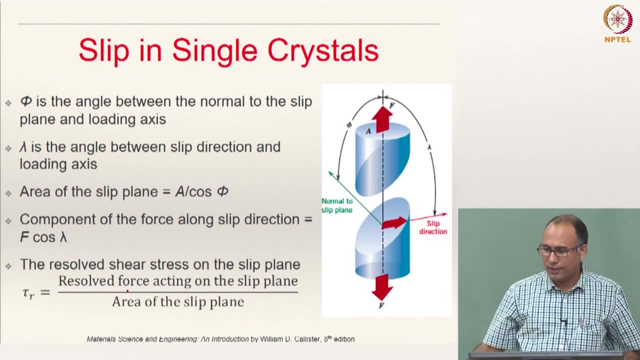 amount of stress. So that large amount of stress, that is, shear stress, depends on the applied loading load or applied stress and the load. So let us say this is a single crystal material and then you are applying a tensile load And let us say that this is the plane on which you want to cause. you want to understand. 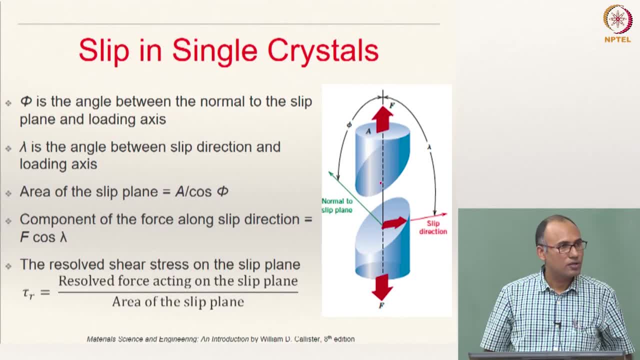 what happens on this plane with respect to the slip. So now let us see that, let us define this angle 4.. The angle 5, the angle 5 is the angle between the loading direction and the slip plane, normal or whichever plane that you are interested in, that normal And in that plane you have. 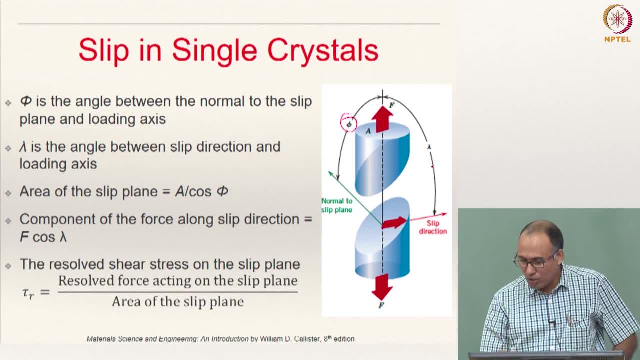 the slip direction. Let us say this is your slip direction. The angle between the applied load and the slip direction is lambda. So p is the angle between the normal to the slip plane and the loading axis. Lambda is the angle between the slip direction and the loading. 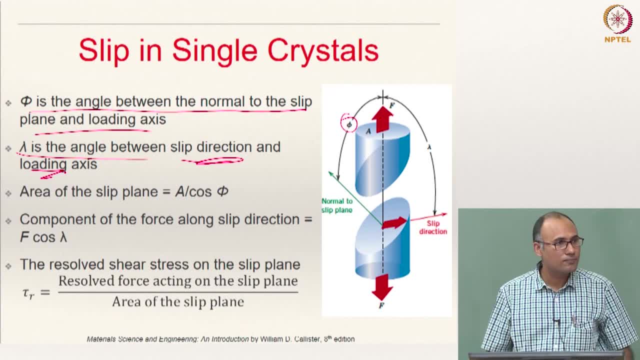 axis. So lambda can be here. i north 6 as 2.. So this is your slip on one忙 And lambda can be here both gradually. So theende is u easily go there. But just remember one thing: if the area of the slip is u 1, so x. 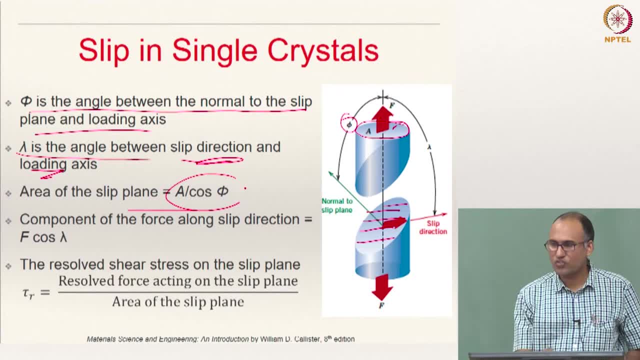 to the power 5.. Now, keep in mind the professors d algebraic aren't Game of human brain and their Paint it table. I am going to mention them. Feel wrestle, But is that clear? Is there any issue there? That is all that we have defined Now. 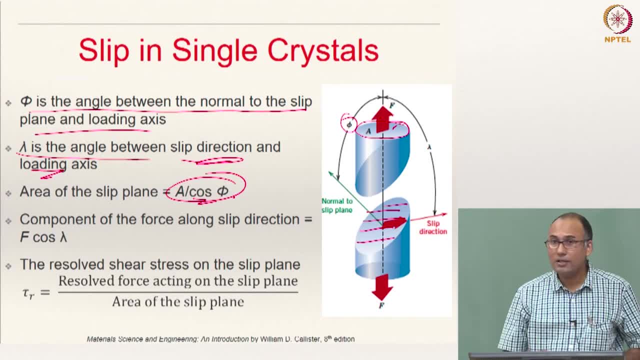 what is the area of the slip plane? If your cross-sectional area of the plane along which the load is applied, if this is A, what will be this area? because this normal angle with That is the area of your slip plane in which you are expecting the slip to happen. 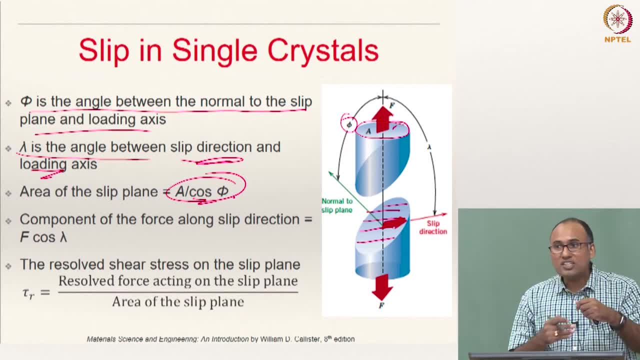 Is that clear? And now, what is the component of force? You are applying a force F in this orientation. What is the component of this force in the direction in which your slip is happening, And that will be the resolved force. The component of that force acting on the slip, along the slip direction, is F cos lambda. 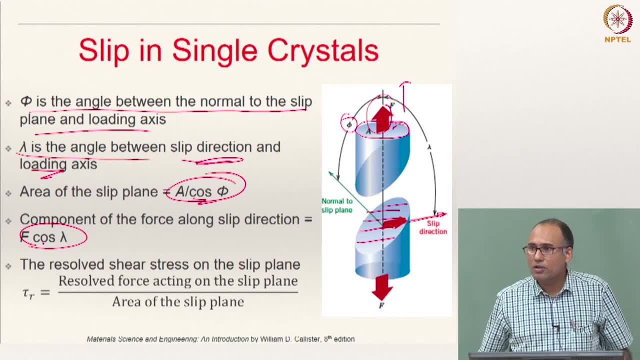 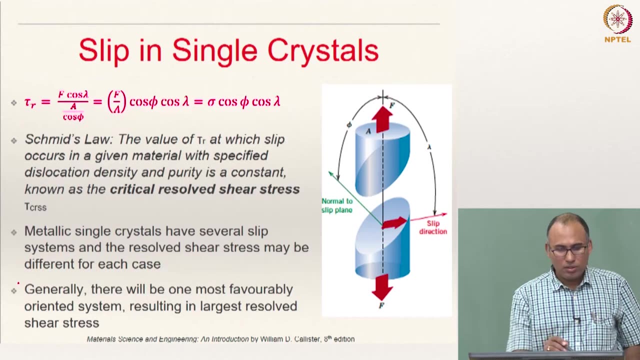 Now, if you have to calculate the shear stress, then resolved force acting on the slip plane divided by the area of the slip plane, That is what you call your resolved shear stress. Is that clear? So now, this is your resolved force acting along this direction. 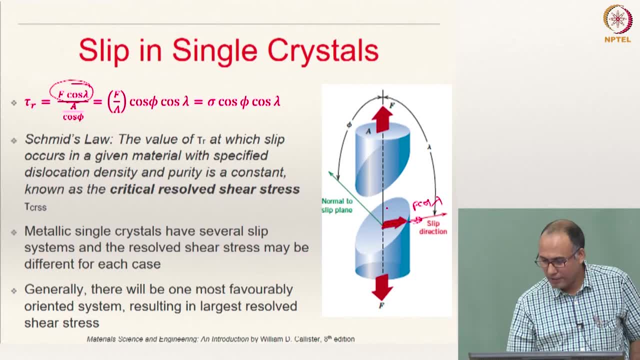 That is your F, cos lambda, divided by the area. Area is this: And that is A by F, cos lambda. That is your area of the slip plane. Then your resolved shear stress is F by A, F divided by this A. A is your area of the. 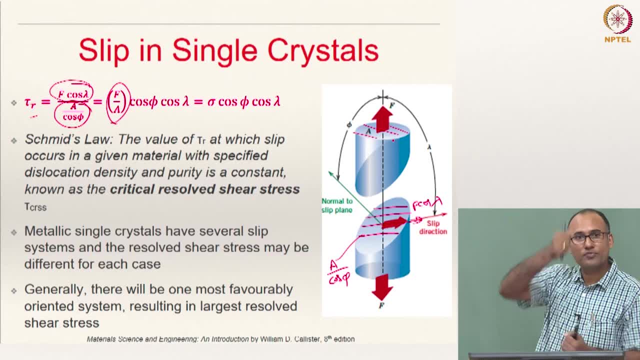 plane normal to which you are applying the load. Then F by A, I denote with sigma that I call applied stress. Then sigma cos, p, cos, lambda. So now we defined What Sumbla called Smith's law. What it says is that the value of tau r or critical, resolved shear stress at which slip 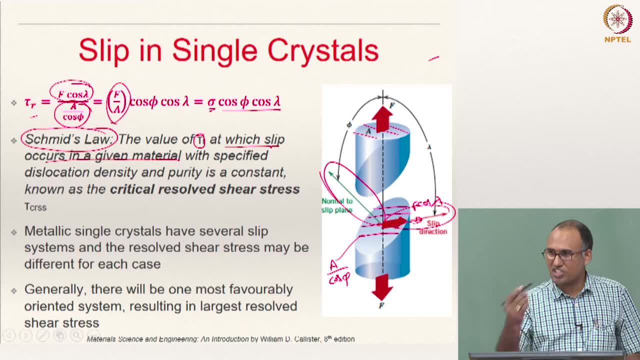 occurs in a given material with specified dislocation density, some initial dislocation density and purity is there The value of the shear stress at which slip occurs and that value is called critical resolved shear stress And that is the material property Right For any crystalline material. 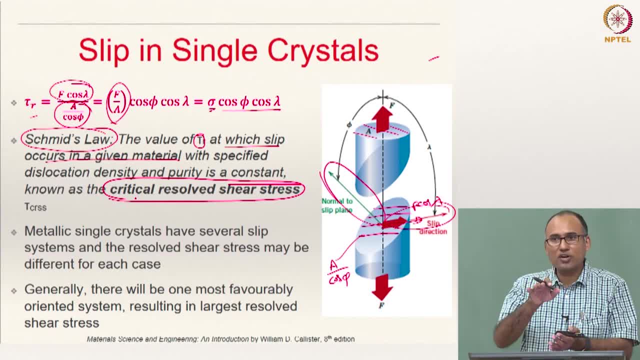 Right. What is the critical? resolved shear stress. That is, the shear stress at which your slip in the material occurs or initiates. It is like your yield strength of the material. It is a material property where you have learnt in your applied mechanics laboratory. 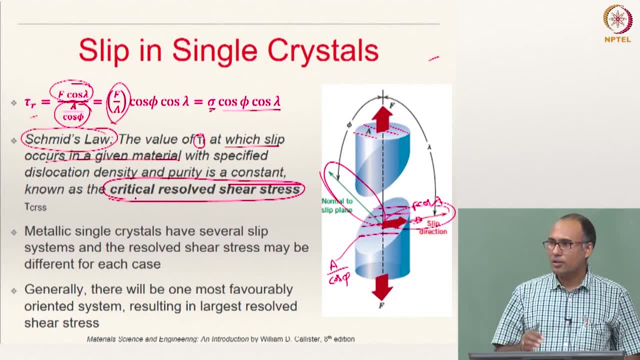 Here we are defining something called critical resolved shear stress, because we are actually talking about shear stress which is causing the slip to the atom. Right, And we know that metallic single crystals have several slip systems. Right, You have several slip systems And the resolved shear stress may be different for each of these cases. 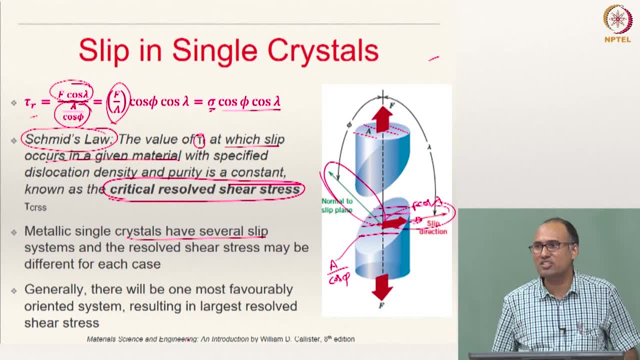 Not all the slip systems will have same resolved shear stress. Each resolved shear system may have different resolved shear stress because we have seen in BCC there are about 48 slip systems and each one of them will have different resolved shear stress because the directions are different. 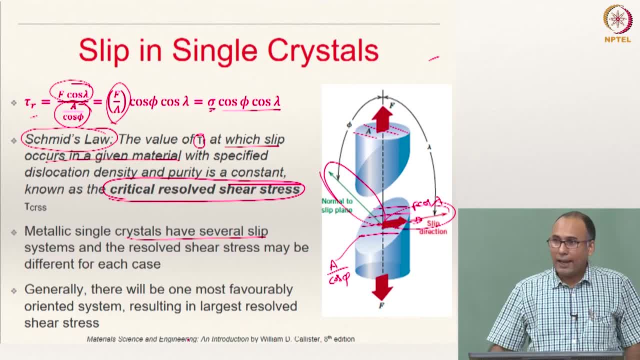 Right, And in general, what happens is you have several slip systems that are possible. Some of them are favourable, some of them are not so favourable, Right. So generally, there will be one most favourably oriented slip system Amongst all the slip systems that are sitting there. there will be at least one in general. 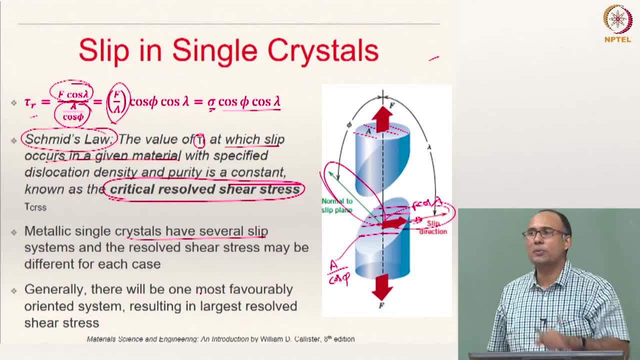 there will be one favourably oriented slip system along which slip takes place. Right Why? Because when do you call a particular slip system is favourably oriented When the resolved shear stress on that slip system is maximum compared to all other slip systems. 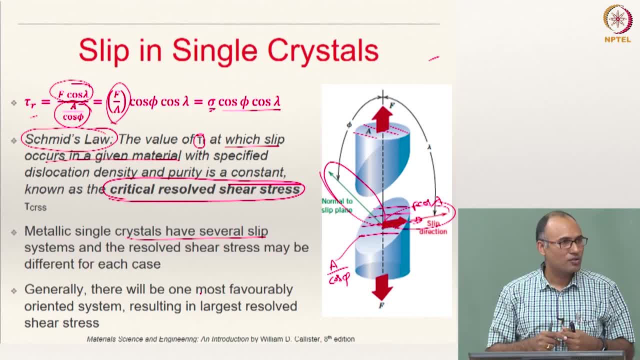 If that is maximum, that means that is close to your critical resolved shear stress. So when your resolved shear stress becomes equal to the critical resolved shear stress of the material, that is when slip occurs Right. So in principle you can have several slip systems and all of them may be active. but 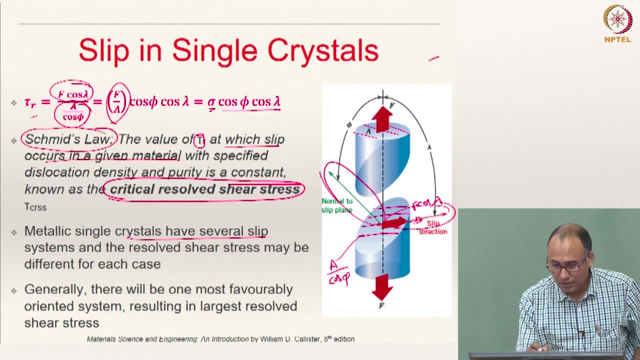 one of them is more active. So that means if you are calculating the sigma is same on all of them. but this quantity, cos phi, cos lambda, is the one that determines the magnitude of the resolved shear stress on that particular slip system. Right, This factor is called Schmitt factor. 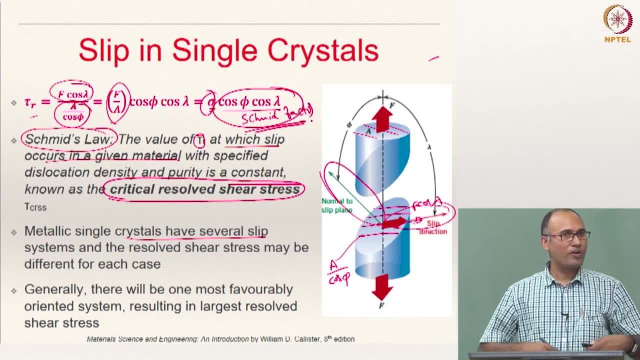 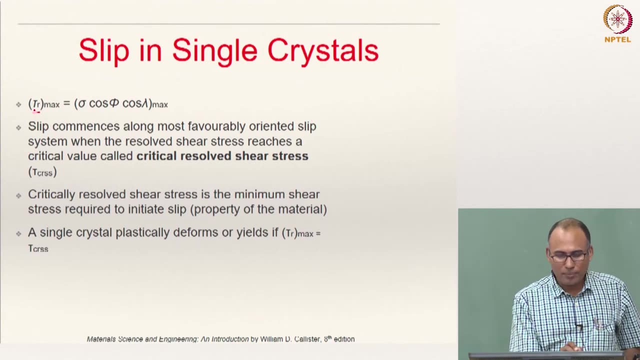 So you need to. your favourable slip system is the one which maximizes your Schmitt factor, So that your resolved shear stress is maximum Right. So the maximum value of tau r, tau r max is equal to sigma, cos, phi, cos, lambda max. 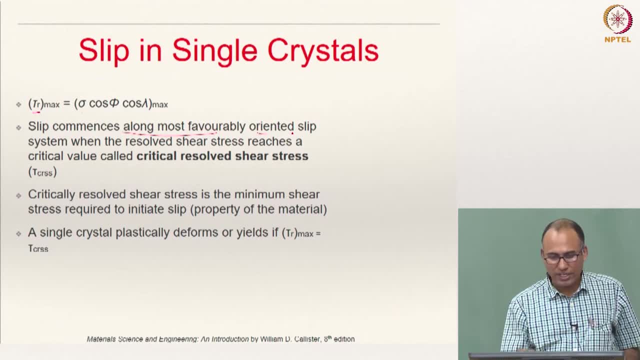 And we know that slip commences along most favourably oriented slip system when the resolved shear stress reaches a critical value called critical resolved shear stress, And the critical resolved shear stress is the minimum shear stress. The critical resolved shear stress is the minimum shear stress required to initiate slip. 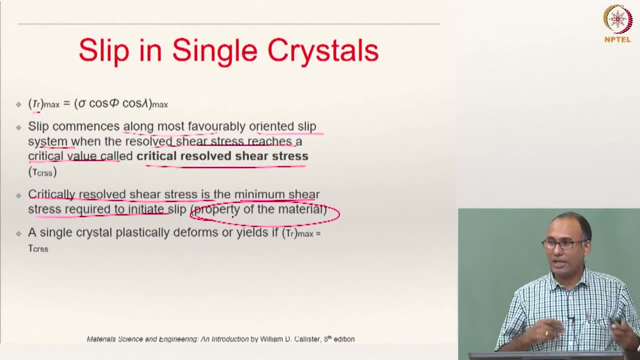 And that is the property of a material. So a single crystal plastically deforms or yields when tau r max in a crystal lattice equal to tau r CRSS. CRSS is critical, resolved shear stress. So now you can write your yield strength of the material. 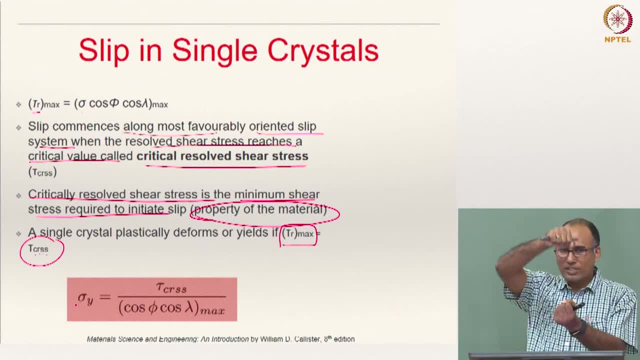 Sigma is your normal stress that you are applying. If you are doing this experiment, uniaxial tension experiment on your, on a single crystal material, as opposed to what you have done on a poly crystal material, then the yield strength of the material will be tau CRSS divided by cos, phi, cos, lambda, max. 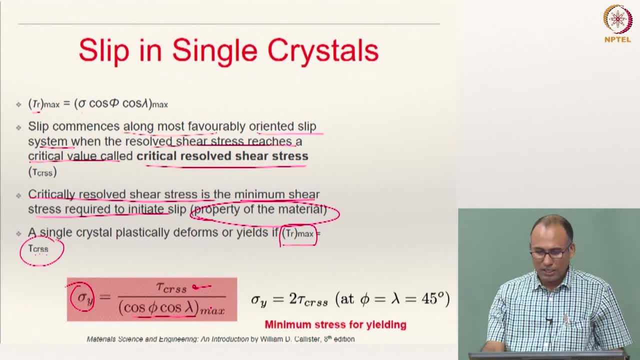 What will be this value? What is the maximum value of cos phi, cos lambda? So the when p equal to lambda, equal to 45 degrees, that is when this quantity will be maximum. That means your yield strength of a single crystal material will be two times the critical. 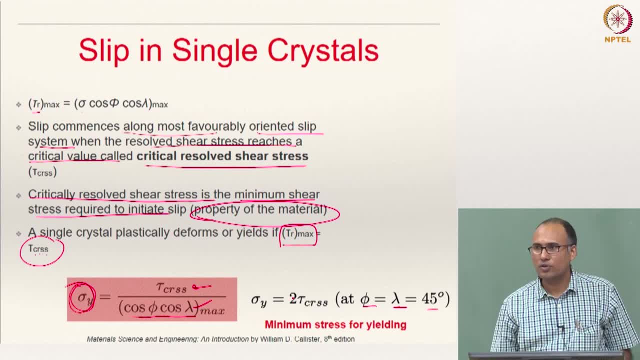 resolved shear stress of this material. You can actually show that the yield strength- yield strength is a normal stress that you are talking about of a single crystal material- is two times the critical resolved shear stress. But one of you can use either this as your property or this as your property- both is. 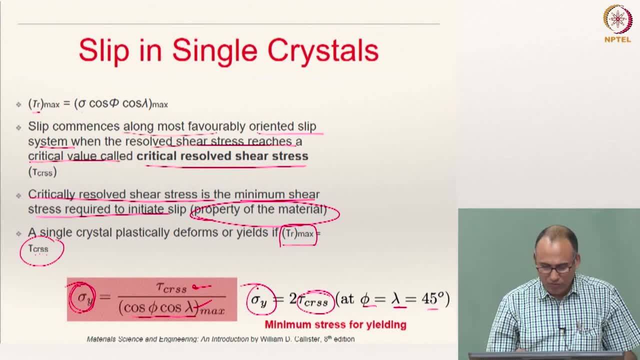 there is a correlation between these two things. that is all, Because this is what we are applying. Okay, This is not what we are applying. This is the resolved component of that, Okay. So, and hence, if you apply a load in the normal direction to the along the axis of 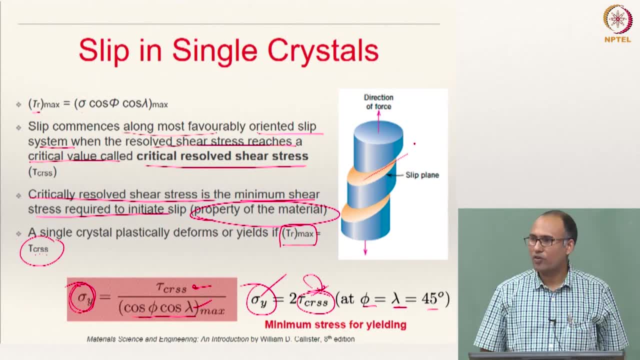 the cylindrical specimen, then your slip tends to happen at 45 degrees And if you see a single crystal material, it is a slip in zinc, single, single crystal. you can see the slip bands nicely coming up. So these are all these. 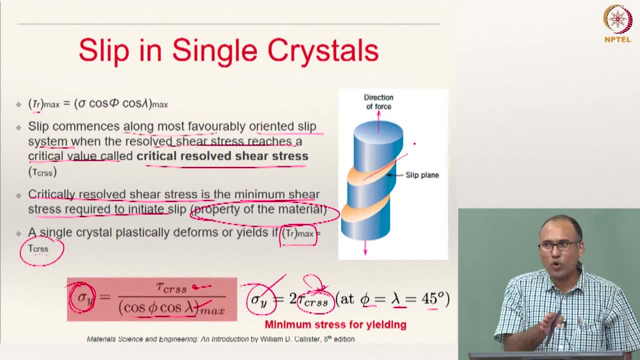 Right. In simple level ofkm evaluation of 행복 slotThe number of Fourier lengths in a continuous gelth gear is the about 26 percent. It is very elegant, Is that everything? Yes, And is there some explained this? Well, there is. Is it? Yes, there are several, without restricting Right. So what is that question? Is it very much? It looks like. it is very useful to look at it in a guided shape, Otherwise this cannot be done. the Kepler process and that one will come after. but there is another question which is none that is necessary. 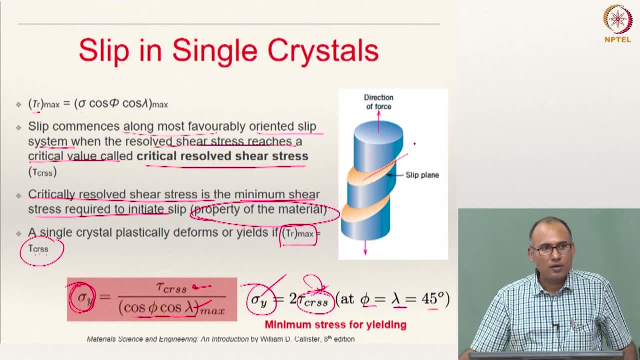 After discussing that dislocations prefer to move in close pack directions, in close pack planes, along close pack directions, we have also discussed about different existence of different number of slip systems in different crystalline crystalline materials. for instance, FCC material has different number of slip systems, BCC has different and FCP has different. 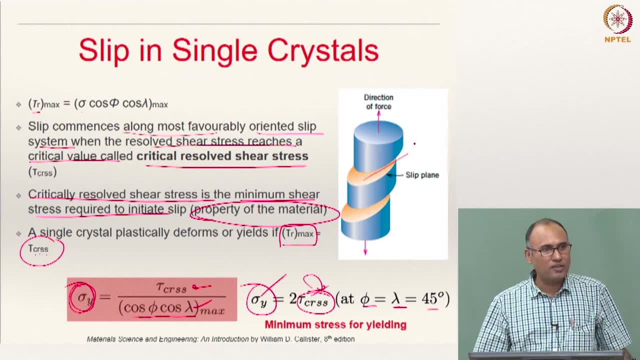 number of slip systems. and then if you are applying, if you are taking a single crystalline material and if you are applying an uniaxial load on the single crystalline material, then you have derived something called critical resolved shear stress. and then we have argued. 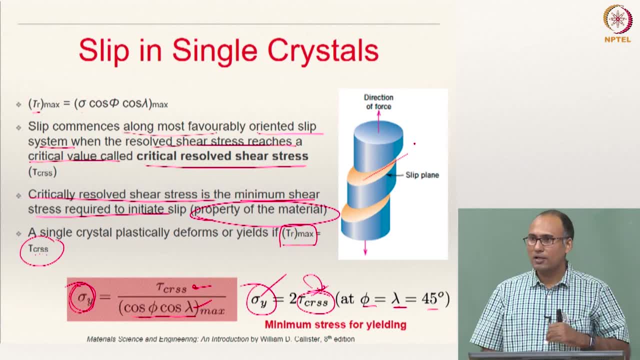 that when this critical resolved shear stress reaches a property of the material called sorry, I am sorry when the resolved shear stress, the resolved shear stress, is the shear stress resolved on to the plane in the Slip direction from the applied load. when this resolved shear stress becomes equal to 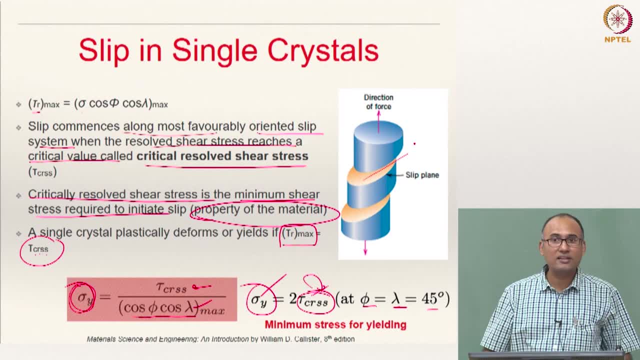 the property of the material called critical resolved shear stress. that is when slip initiates, and we have actually derived the expression for resolved shear stress. and then you should be suppose, if you know what is the load acting in a particular direction, you should be able. 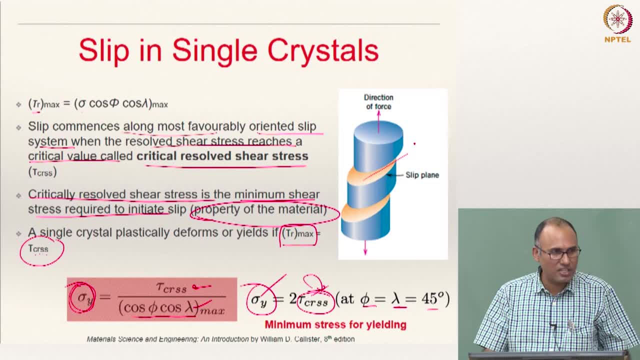 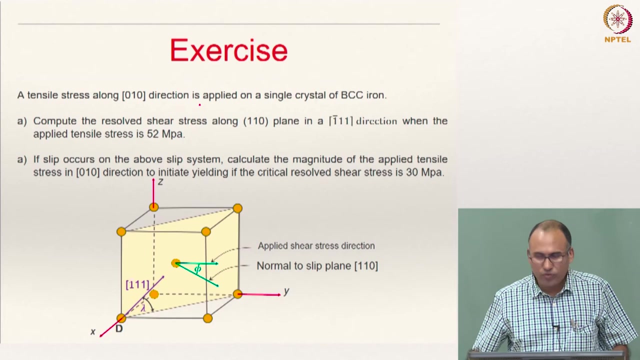 to calculate what is the resolved shear stress in this material, in that particular shear stress in particular place. Now we have similar铆 theikal motor anymore cuánt or millinspire zone. well, this will also be…. You will carry out the�� Flower system exactly from other首. 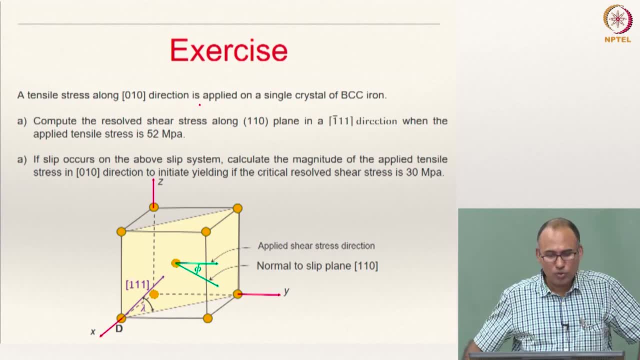 Slip System and then, if you know the critical resolved shear stress of the material, you will be able to comment whether the material is yielding or not. fine, That is where we stand until now, So it may be a good time for us to solve this problem. 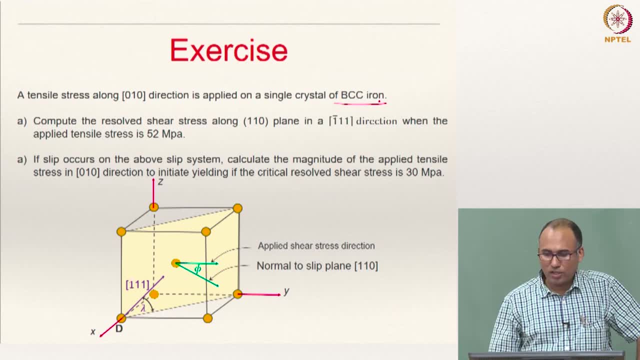 You have a single crystal material, which is BCC, iron, iron. If you have just one cut and then if you use the distance between the next two, you will be able to handle this problem, And on that you are applying a tensile stress along 010 direction. What is 010 direction? 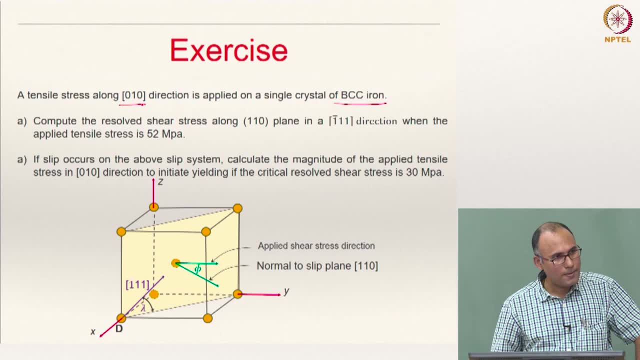 here. That is your 010 direction, Is that correct? And now, so that is, this is also 010.. In that case, this is 010 direction. Agreed, And compute the resolved shear stress along 110 plane. What is 110 plane? That is your 110 plane, right? That yellow one, this? 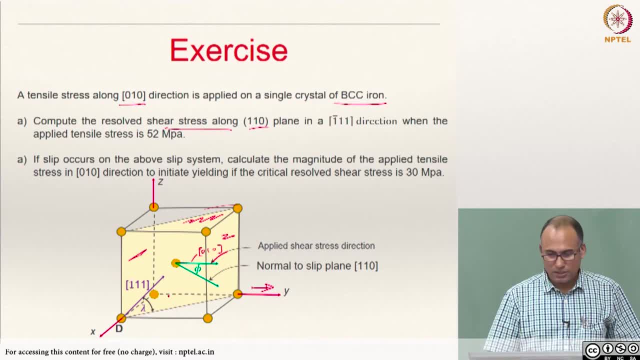 is your 110 plane, is not it? So you need to compute the resolved shear stress in 110 plane in 1 bar 1, 1 direction. Where is 1 bar 1, 1 direction? That is the body diagonal right Connecting the body diagonal. Is that correct And that? 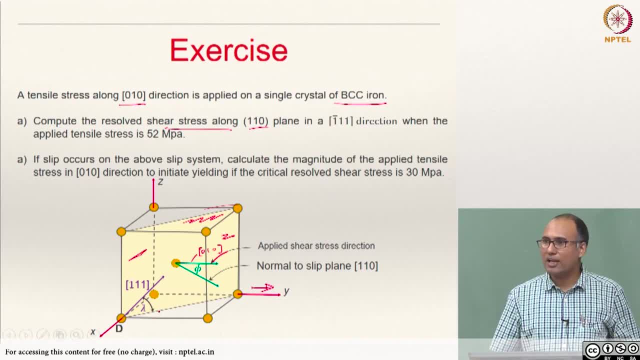 is your 1 bar, 1, 1 direction. So you need to calculate the, now the resolved shear stress along that direction in this plane. How do you calculate? First you need to know we need to calculate the resolved shear stress along 110 plane, So you need to calculate. 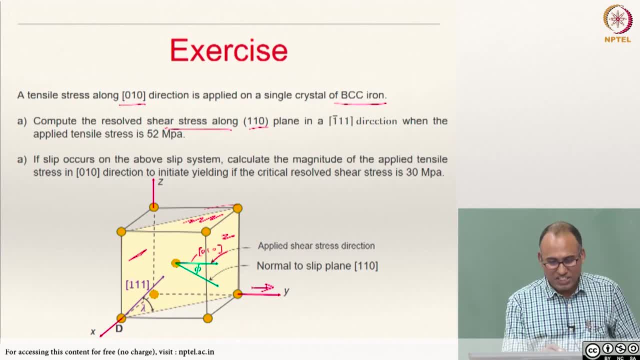 Smith factor When the applied stress is 52 MPa. So we have this formula Resolved. shear stress is equal to sigma, cos, P cos lambda. Sigma is given as 52 MPa And P is what The angle between the force and slip direction. right. 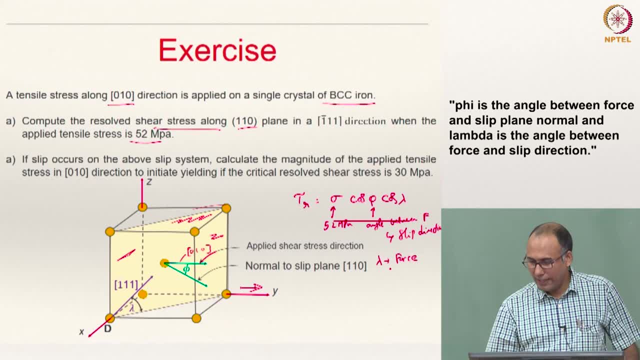 And lambda is force and slip plane normal, is not it? So what is the direction of the force? This is your direction. vector Force is acting in that direction. And what is the normal to the plane? Normal to slip plane is 110.. That is what he said, right, Because 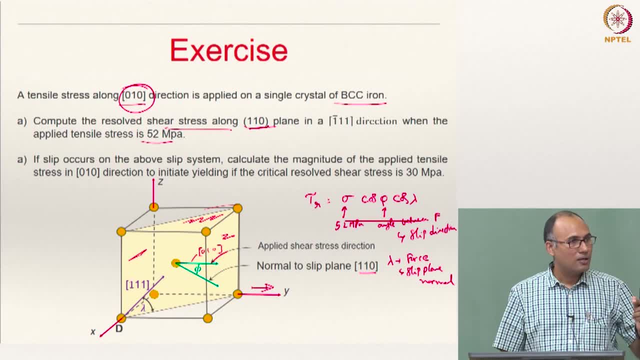 it is a cubic crystal. So you need to calculate the resolved shear stress along 110 plane. If it is 110 plane, the normal to normal direction also will have the same indices. That is what we have discussed. If the plane is 110, in a cubic crystal, then the normal to the plane. 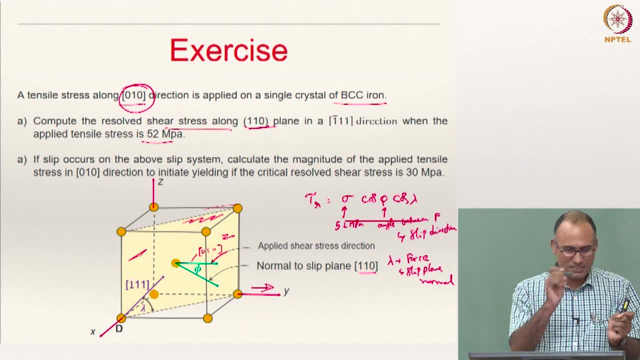 the direction vector will also have exactly the same indices. So this 110 plane will have a normal in 110 direction. right Now you need to find the angle between 010 and 110.. So you need to calculate the resolved shear stress along 110 plane. So you need to calculate. the resolved shear stress along 110 plane. So you need to calculate the resolved shear stress along 110 plane right, Siffer by completeness right, Siffer by completeness right, And to establish the pled shear stress along 110 plane. now it should be 0.. 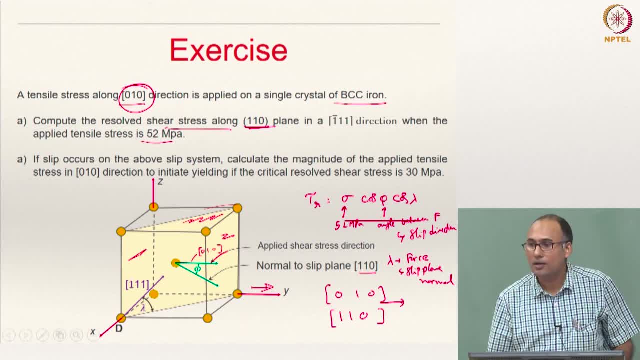 And now, if you pester the shear, what will it give? right, The sample professor will give you what. What will it give? Pi or lambda, Louder Applied force and the normal Pi or lambda? Dakshita Chopra and John Cochran. 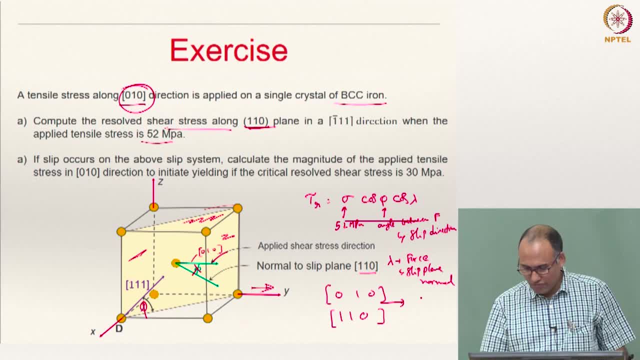 And this is. this should be pi, and that should be lambda, right? So now you will get pi, and then again 010 and 110, Metho, right? Yes, That means that you have to calculate twice to be a laughing particle, right? 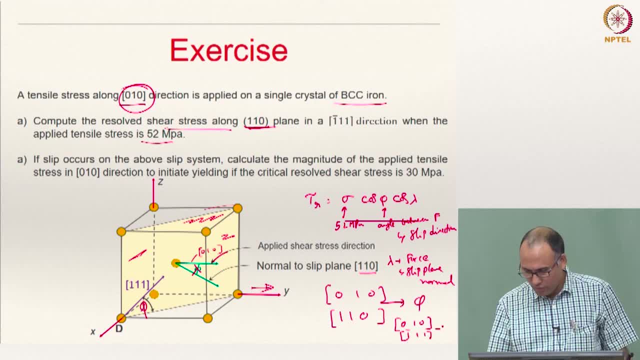 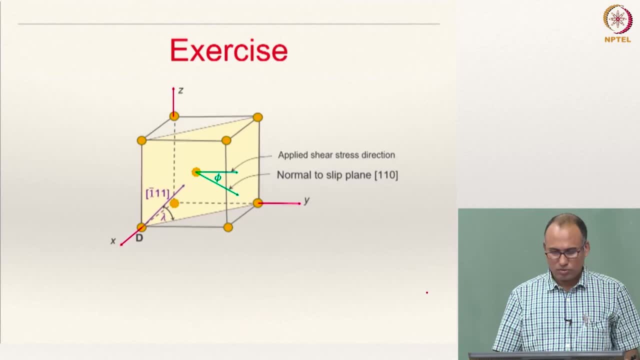 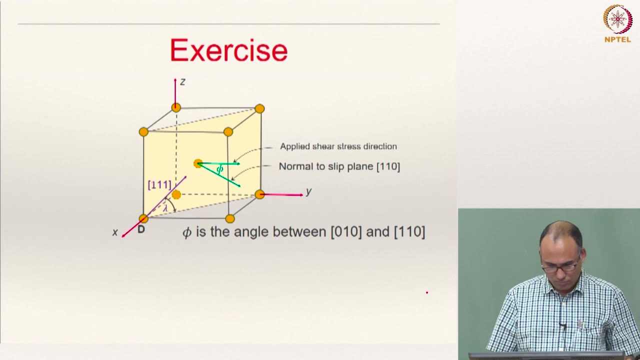 Positogiали, I have tried. have I, among others, have I seen twice Say this chord: 1 bar 1, 1 will give you lambda. You know how to calculate this phi and lambda right, So that elementary vector algebra. you will do that. and then phi is the angle between: yeah, 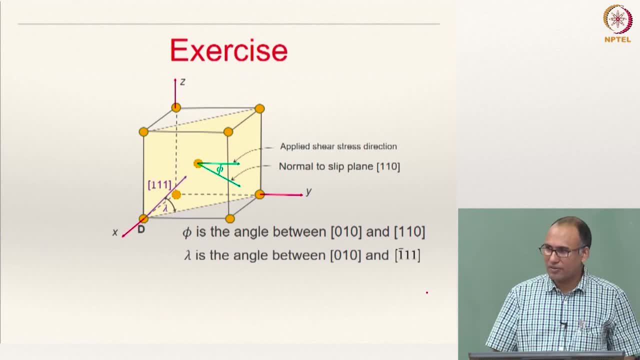 I made a mistake, but does not matter. okay. Lambda is the angle between that, and then the OR is equal to sigma, cos, phi, cos lambda, and here phi. the angle between these two guys is 45 degrees and this is 54.7.. So the resolved shear stress is 21.3 MPa. You are 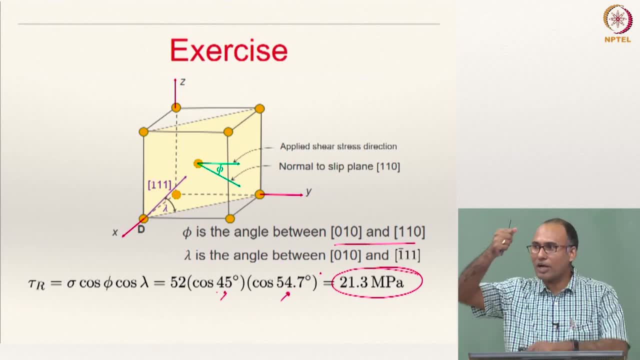 applying 52 MPa, but the resolved shear stress on that particular plane is 21.3 MPa and if you change the direction, instead of 1 bar, 1, 1 direction, if you choose in another direction, this value will change right. That is natural. 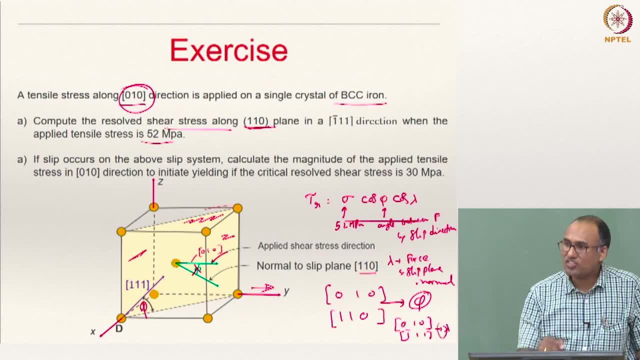 And now the second question is: if slip occurs on the above slip system- let us say the slip is occurring- Calculate the magnitude of the applied tensile stress to initiate the yielding. if the resolved shear stress is 30 MPa, because 23 MPa is the resolved shear stress if you are applying- 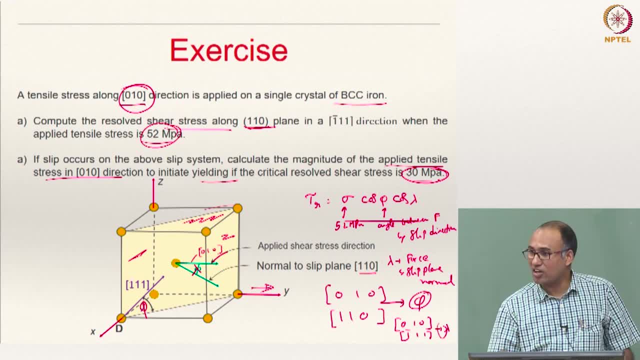 52 MPa. That means if the critical resolved shear stress is 30 MPa means it is not actually yielding because the resolved shear stress is less than the critical resolved shear stress. Now, if you have to import slip, then what should be the stress that you need to apply?